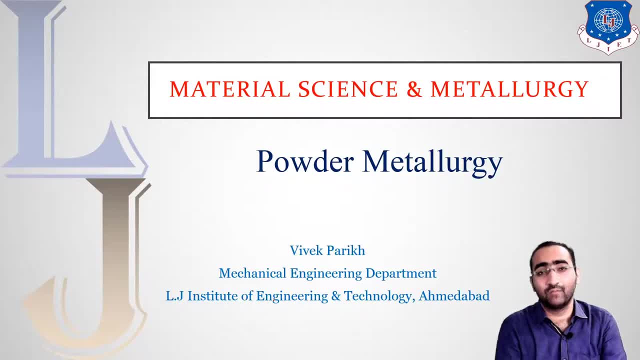 the steps of the powder metallurgy and in that step we have discussed the first two steps, that is, the powder production methods, and then we have gone for the second step, that is known as a particular step, that is the powder conditioning step which comes, that is, the mixing and blending of the material. we have done 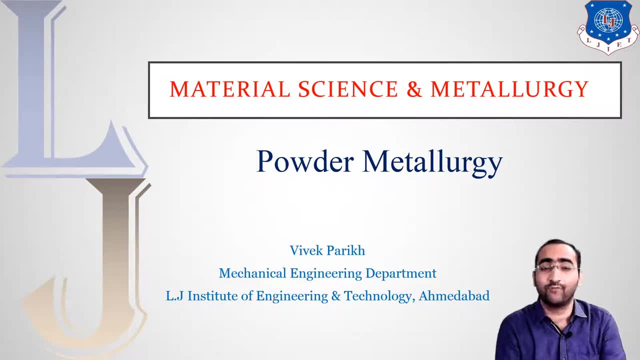 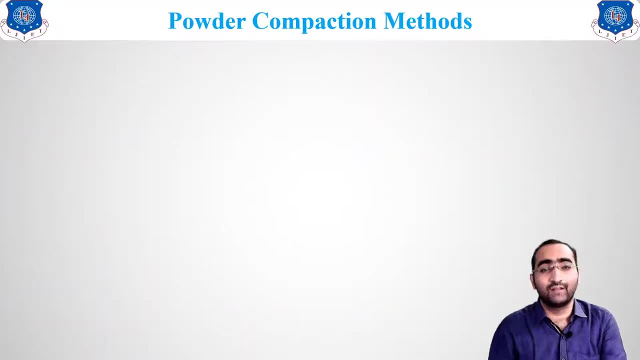 That means the powder has been prepared and now it is ready for getting into the shape. So what we are want? we want a proper shape of the material. So for that we will be going for our third powder metallurgical step. that is known as. 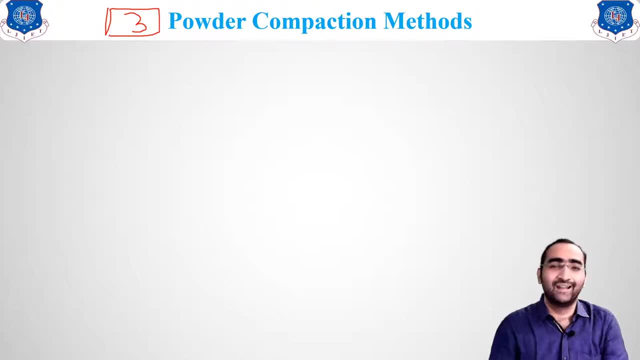 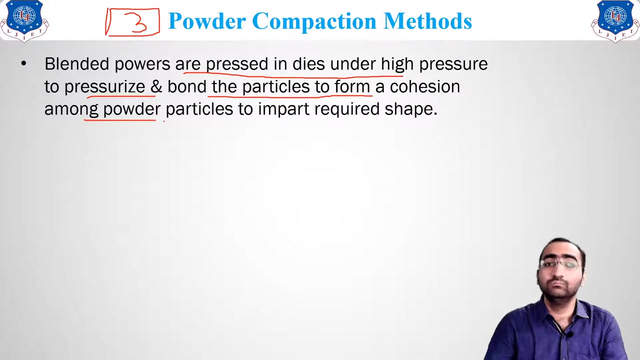 a powder compaction method. Okay, so let us start about the thing that is known as a powder compaction method, Now blended parts. they are then pressed in dyes under a high pressure to pressurize and bond the particles. to form cohesion among the powder particles to impart the required 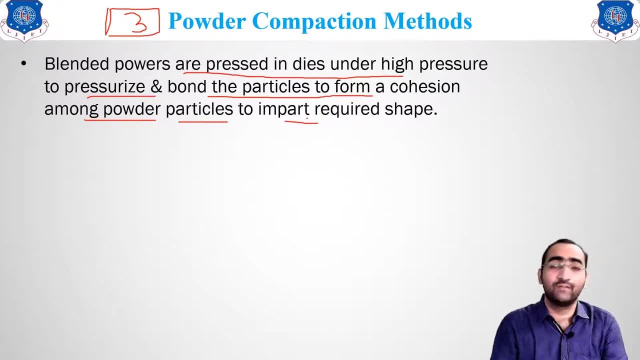 shape. So the blended particles. what we are doing, we are applying the pressure on it and, as a result, we will be allowing it to get the final shape of the material. So to work the part after compaction, whatever the after compaction we are getting, that is. 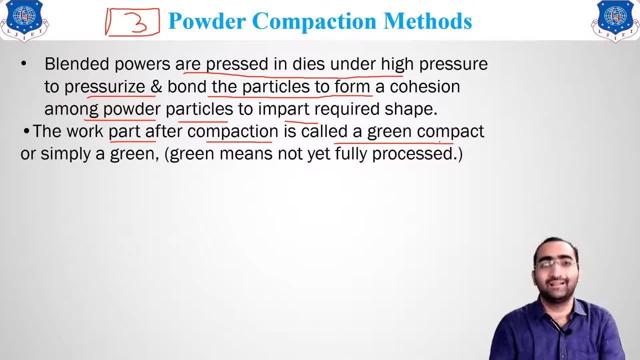 known as a green compact, whatever the thing. take a sand, take a clay- okay, sand after adding water. what will happen? clay after that, clay you take or you give that particular thing. that is a ball shape. whatever that ball shape you are getting, that is known as a green material. 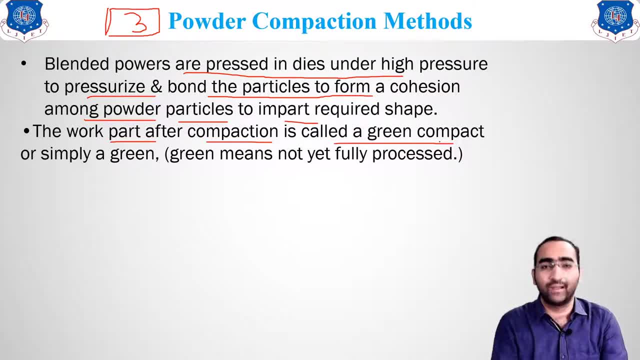 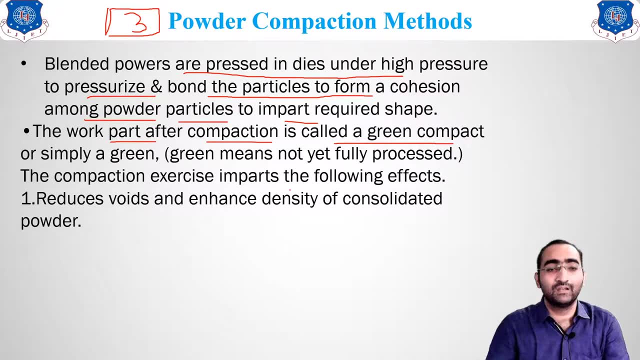 or you can say the green, simply green, green, compact, clear. So the compaction exercise. Why So the compaction for the compact? what effect we will be getting? that means it will, first thing, that is, reduce the void, whatever the gap which are there between the two different. 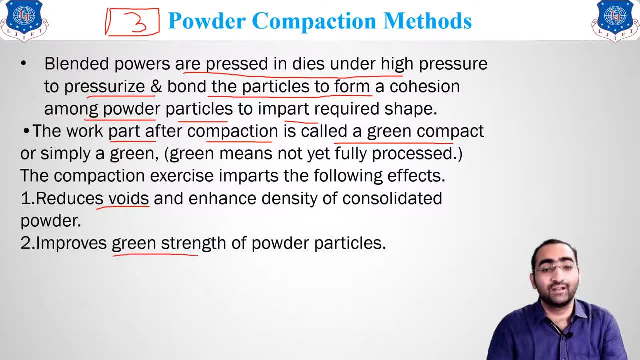 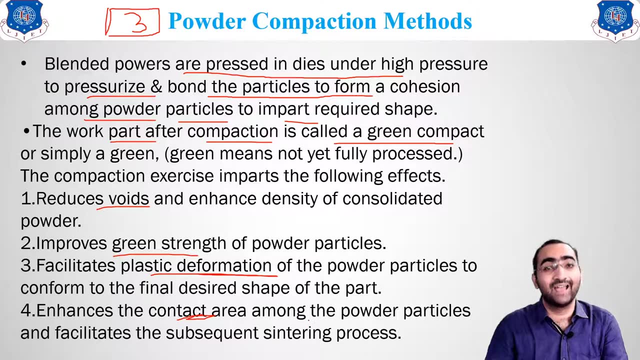 particles. that is getting reduced. second one: it improves the green strength of the particles. third one: due to that thing, what will happen? plastic deformation of the material will be there and, as a result, the final product shape we will be getting. and the last one, that the contact area is less. why? because we are taking that material into the sintering purpose. 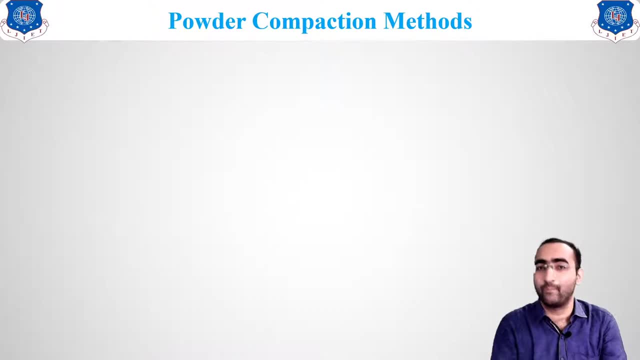 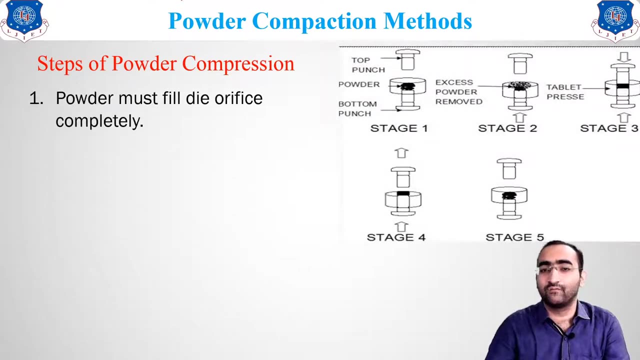 For that contact area is minimum with the help of this compaction. Now let us see how does the thing happen, how the steps are there. these are the different steps you can see over here. the very first step: powder must fill die orifice, completely, fill all the powder fill the orifice. whole orifice is filled with the help of the powder. 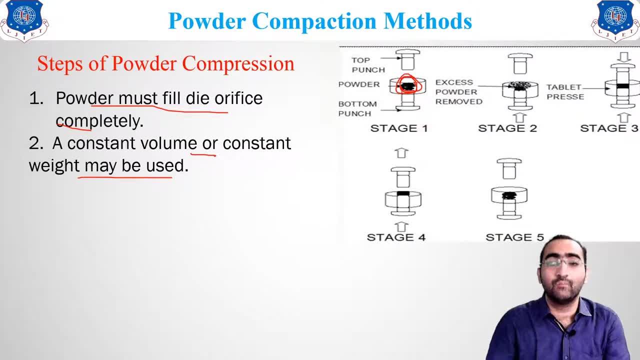 second one: a constant volume or the constant weight may be used. that means, during the all the processes, the whole load or the volume, the constant volume may be used. So what will happen? What will happen? What will happen? constant volume should be taken, otherwise there will be a change in the dimensions, will be there. 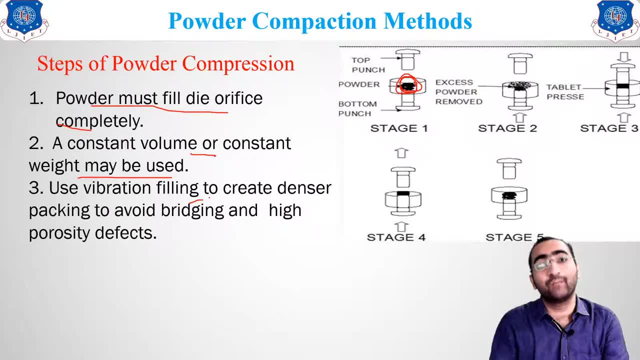 use vibratory filling. what will happen due to that vibratory? the powder particle will get settled down perfectly. if you are not applying vibratory, then there are chances of voids. are there between the two particles? apply pressure along more than one axis to minimize the defect. 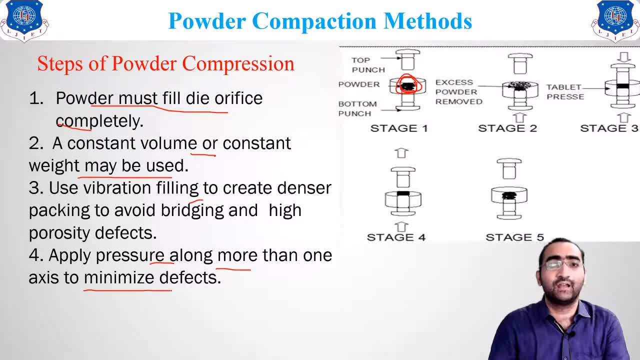 you can go for the one direction, two direction, any of the direction. you can go for the compression. so what will happen? the material will try to compress and, as a result, the shape of the material will be there. after that compression, eject the material, take away the material and repeat the. 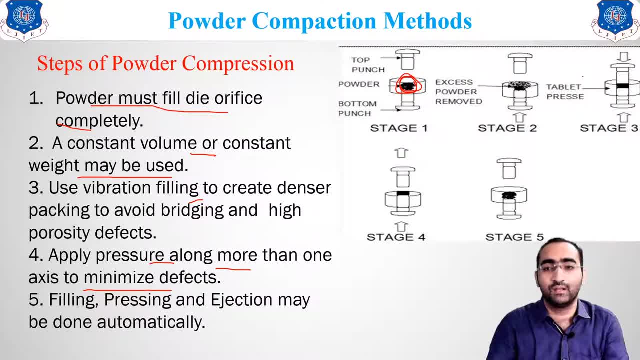 whole cycle. once again you can see over here: fill the material, press the material, remove the punch and after that eject the material and then once again we will be coming back to our first step and in this way we can say that these are the different types of the steps of the powder. 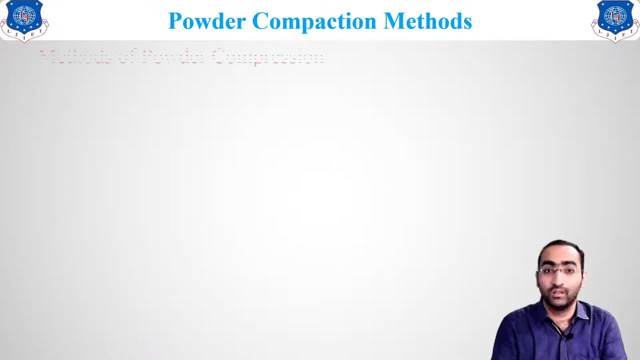 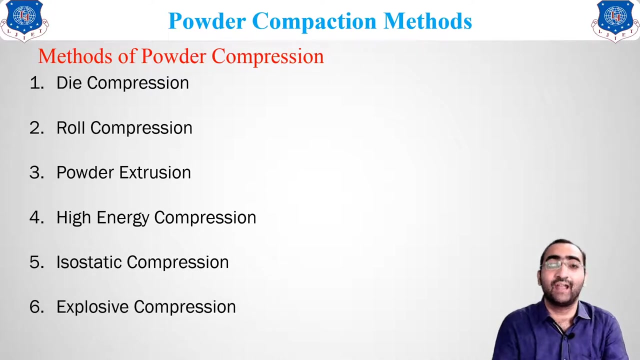 compression, the basic steps of the powder compression. there are many methods of the powder compression. there are seven techniques out of that. the first one, die compression, which we have discussed. second one, roll compression, powder extrusion, high energy compression, isostatic, exclusive and the last one, vibratory compression. let us discuss 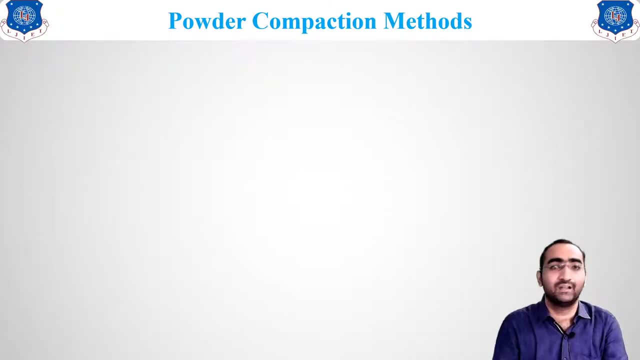 these all the different types of the compression in the detailed one. so the starting with the very first one, that is known as a die compression method. whatever the thing we have discussed earlier during the step, the same thing is applied over here. you can see the figure: the same thing. 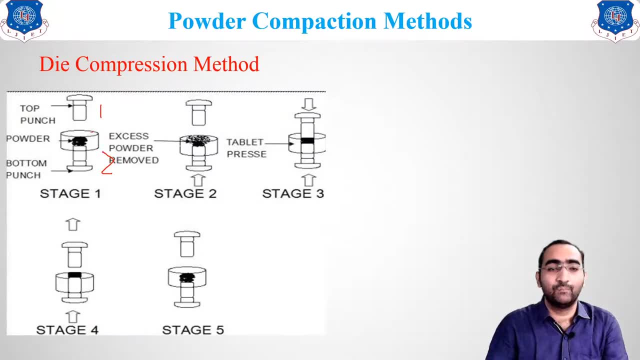 this is nothing but the two die. two dies are taken between. that powder is allowed to praise and that is known as a die compression method. metal is allowed to compress between the dies and then brought into the shape. forces can be applied from one side or you can go for the both the sides. it is. 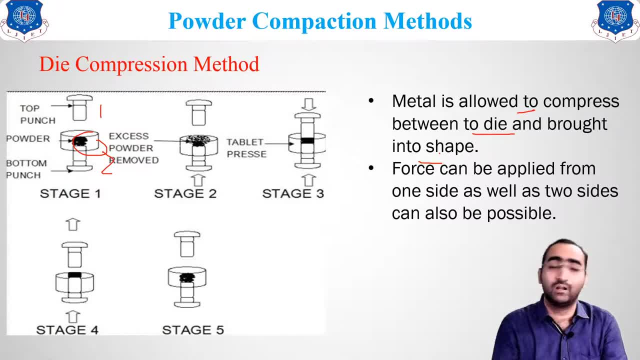 up to us how we are going to apply the pressure on the material. it will depend on the material material, which material we are taking. according to that, we will be going for the die compression method. clear. so that was the very first method, the simple method: die compression between the die. 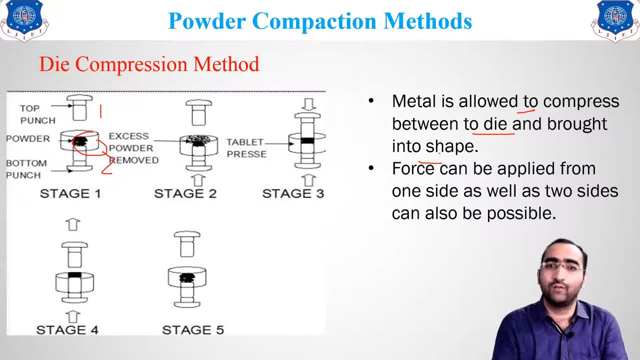 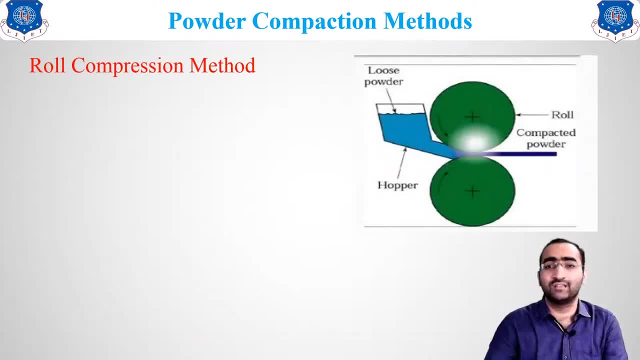 take the powder, press it and due to that pressing, what will happen? we will get the final shape of the material. after that second method, roll compression method. you can see over here, between the two rolls the powder is allowed to place and the powder is moved. due to that thing, you can see. 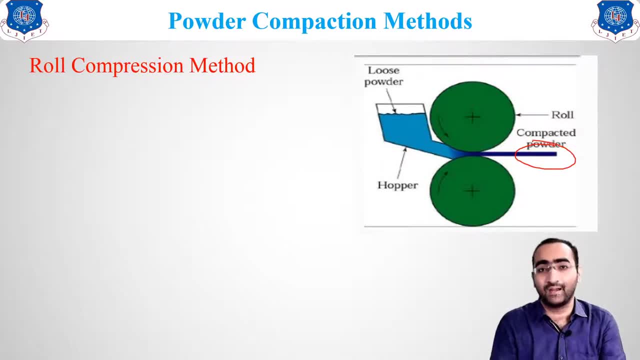 over here the thing that is the compressed part we are getting, where we can use this thing. roll compression method maximum we can use for the manufacturing of the flat sheets, the whatever the flat sheets- a long, very long flat sheets can be obtained with the help of this method. 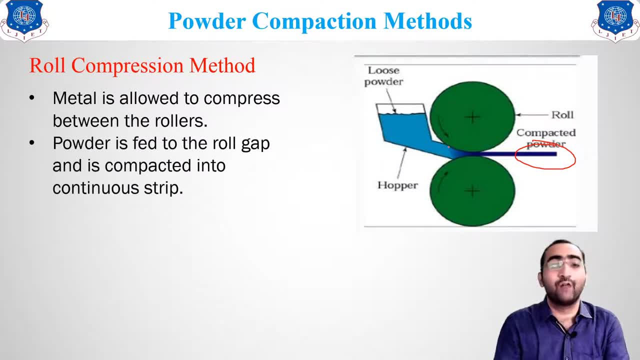 metal is allowed to compress between the rollers and powder is paired to the roll gap. the thickness of the sheet is dependent on this roller gap. so, roll gap, whatever the gap is there between the roll, it will totally depend on that thing. and the continuous strip, continuous long strips, can also be manufactured with the help of this roll. 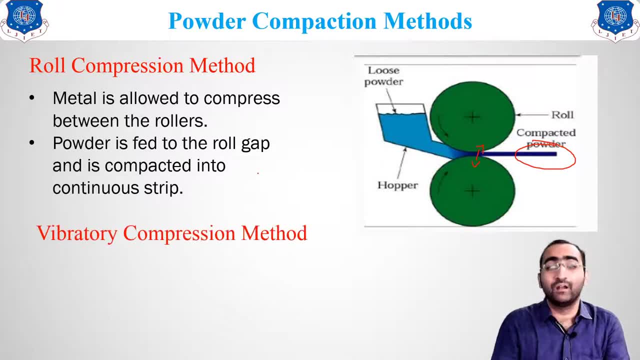 compression method. third method, that is, the vibratory compression method. it uses the low pressure and continuous vibratory motion to compress, the same as the die die compression. but what is the change? that is, the vibration is allowed during the filling. so due to that thing, and the density is more, so strength of the material can be increased with the help of this. 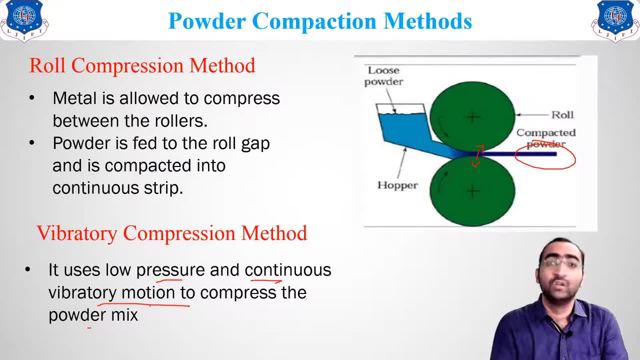 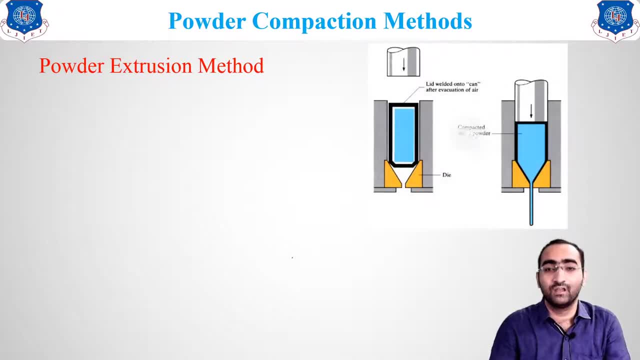 vibratory compression method. okay, so now going for the fourth method, that is, powder extrusion. what do you mean by the term extrusion? you can see from the figure that if the material is allowed to press from the back, what will happen? the material is allowed to move from this thing. 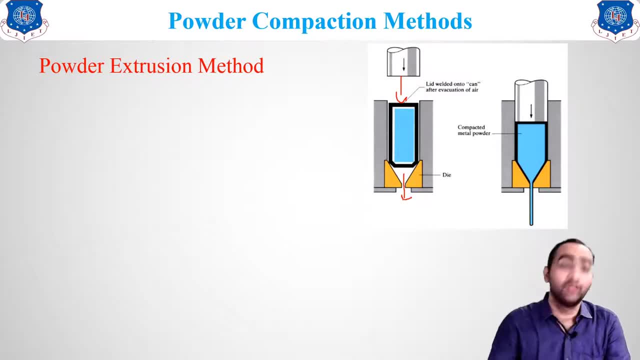 out during the movement of this thing, out what will happen. the material will come out and this is the thing: cylindrical pipes and all that thing. cylindrical part can be easily, a long lasting part can be easily obtained with the help of this method- extrusion method, if you want to understand the 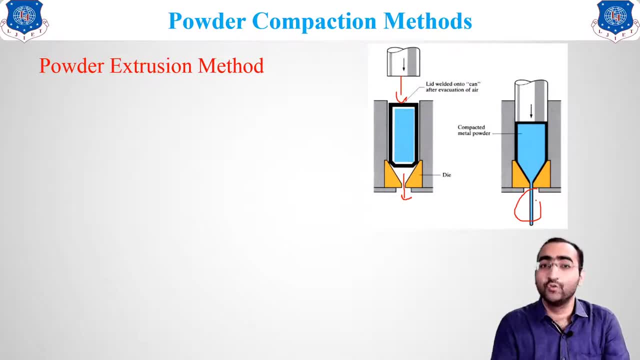 simple method. whenever you are using the paste, you are applying the pressure at the back. what will happen from the top, from the outlet paste comes out? the same applies over here. the metal is filled in the container metal. we are applying the pressure. what will happen from the out outlet? 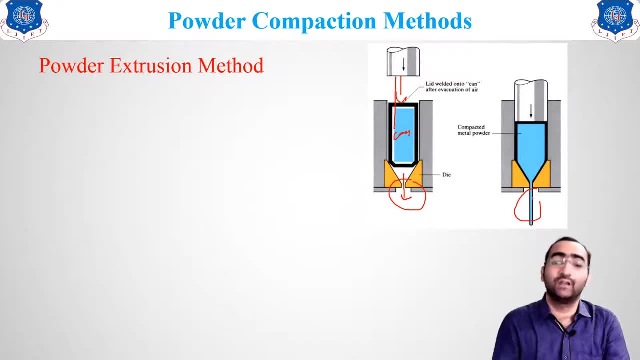 the material will come out in the form of that shape, of that outlet. okay, metal is allowed to compress between the rollers and, due to that thing, powder extrusion method takes place. okay, now comes the next method, that is known as an high energy compression. high energy compression, that is: 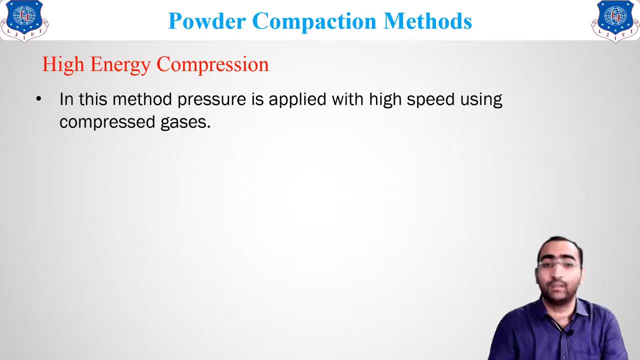 nothing but the method in which we are going for the hydraulic press. the method: pressure is applied with the high speed using the compressed gases. due to that compressed gas is what will happen, as a result of which the compressed gas will be helping for that particular thing. that means a very high 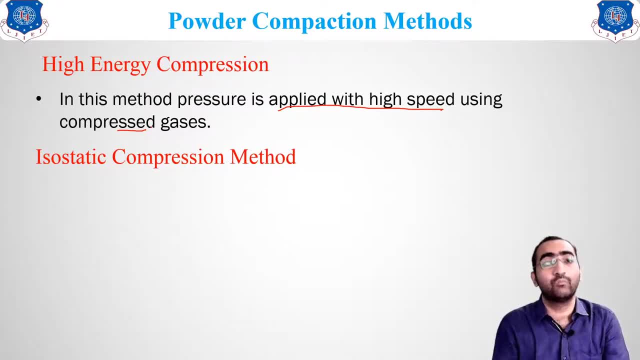 compressed gas will make the metal powder come close to each other and, as a result, you will get the powder compression and the last method, which is there, that is known as an isostatic compression method. in that isostatic compression method, you can see the liquid is filled all around the thing. 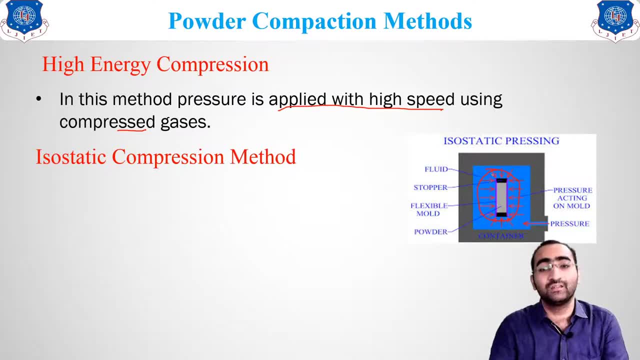 and a proper, same amount of energy or the load is applied on this material. here the powder is filled and, as a result, what will happen? this liquid, by applying the pressure, what will happen? this liquid will transfer the pressure on this material and, as a result, what will happen? 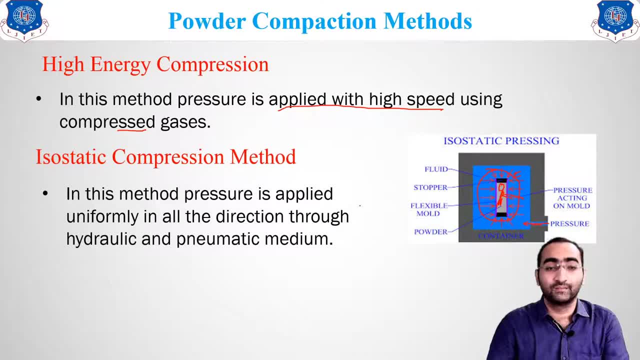 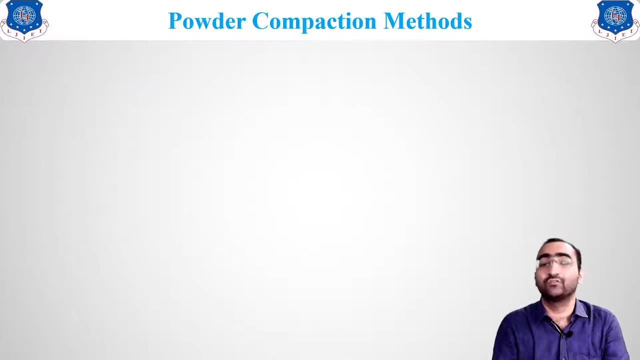 the proper compression of the material will take place. in this matter, pressure is applied uniformly in all the direction through the hydraulic and the pneumatic medium and, as a result, a proper type of the perfect compression has been done with the help of this isostatic thing. 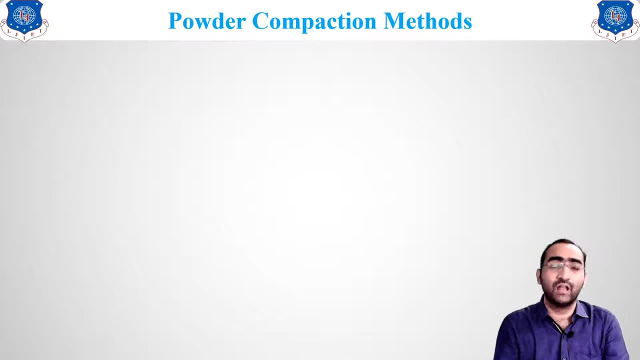 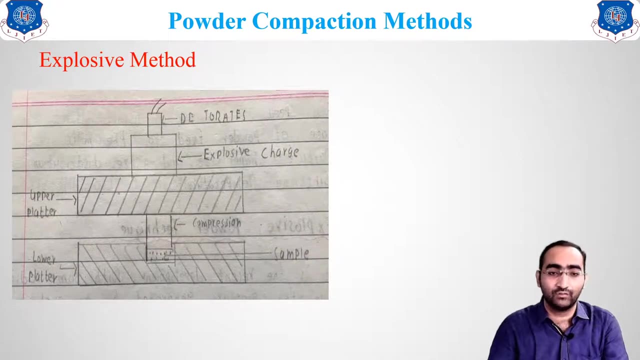 there are certain material which cannot be compared with the help of all this thing, for for that thing there is an explosive methods which we can use. so here you can see, there is a two thing, two dyes are there. so in that, two dyes, what are there? here you can see the upper die. 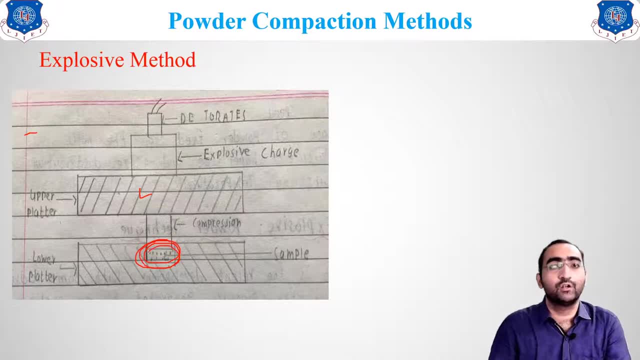 lower die and here the powder of the material to be pressed is taken. above that thing, you can see there is an explosive which is made and that is ignited. what will happen due to that? here the explosion takes place. due to the explosion, large amount of energy is produced and with the help of 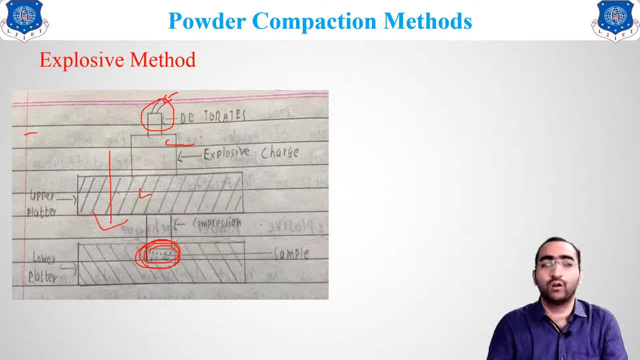 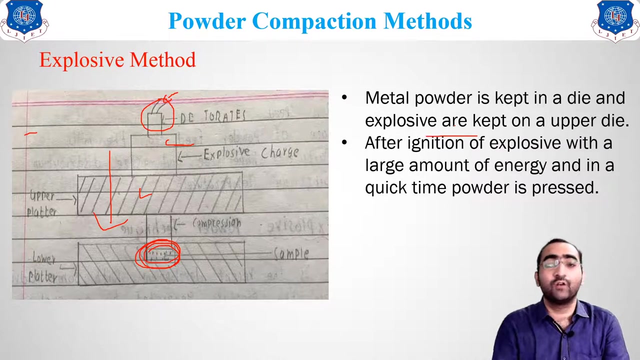 a very high speed this thing comes down and in a one shot this will get compressed. this method is such a method that if you start the method, you cannot stop that method. so metal powder is kept in a die and explosives are kept on a upper die after ignition of the explosion. what will happen? 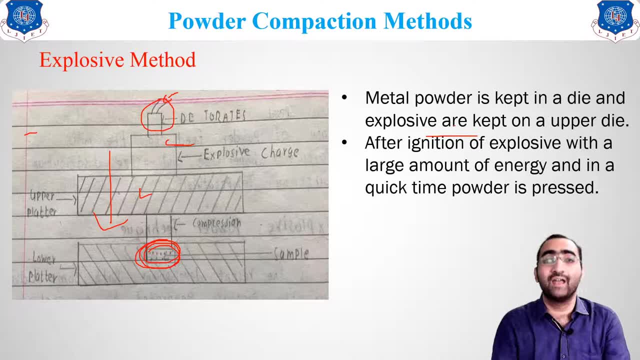 large amount of energy in a quick time is produced and all that energy is transferred to the material and with that, all the force. the material is getting pressed and due to that, what will happen? the powder compression takes place, which are the explosions which we can use. the explosions like 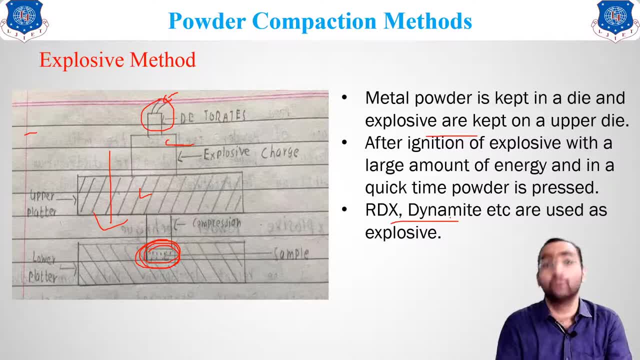 rdx, dynamite, etc. which we can use as an explosive so that it will transfer its energy on the material and the powder compression takes place, clear. so here it ends, your third powder production method. sorry, powder metallurgical match step that is known as in powder compression. so we have generated 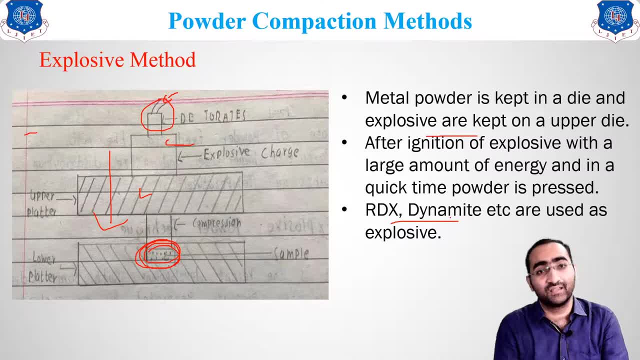 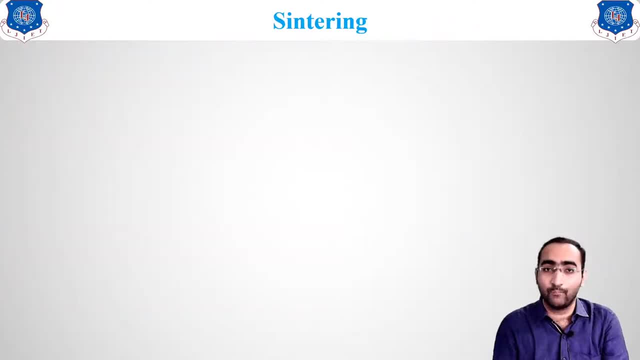 after powder producing, what we done? we have gone for the mixing. after mixing, we have taken it, with the help of the compaction, its shape. so now going for the fourth step, which is the most important step of the powder metallurgy, because properties are dependent on it. that is known as an sintering. 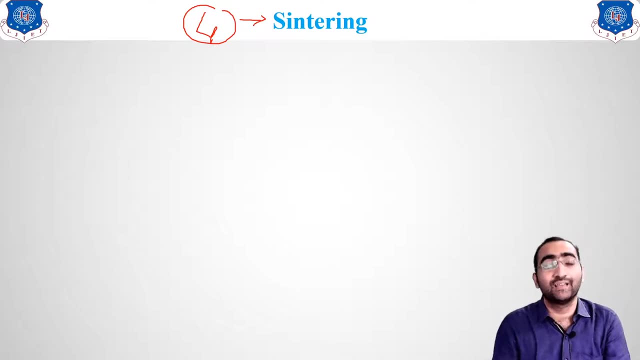 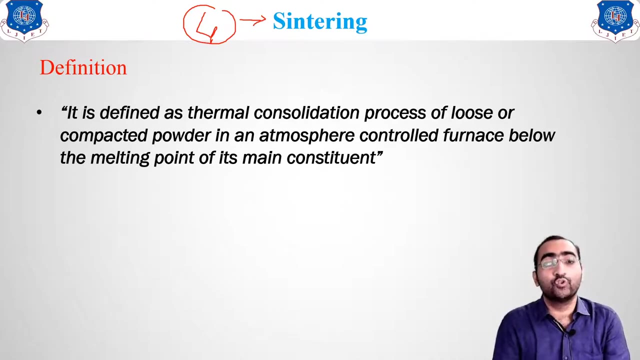 of the material. that particular thing is known as an sintering. now, what do you mean by the sintering? it is the thermal consolidation process of loose or the compacted powder in an atmosphere controlled furnace below the melting point. we are hitting the material in a controlled atmosphere. clear, hitting the material in a controlled atmosphere. but what will? 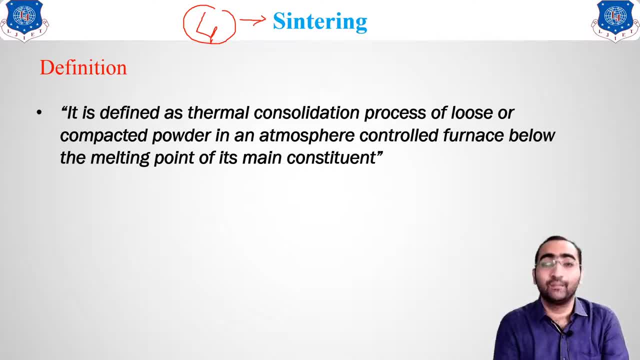 be the temperature. it should be always less than the melting point of the material. if you go for the higher melting point, what will happen? due to that thing? your material will get melted and as a result of which, once again, you have to start from the beginning. clear, so you should take it in mind. 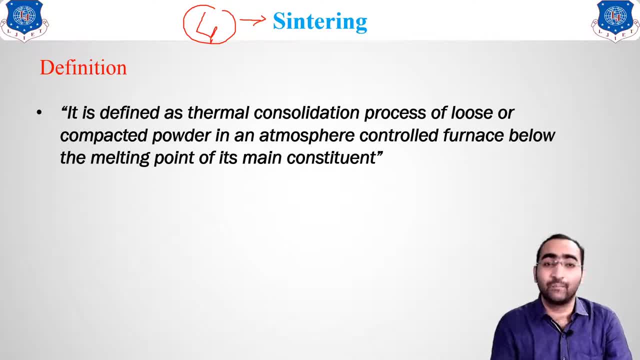 is not allowed to melt, so it should be always less than the melting point of the material. two types of the sintering are there. they are the solid state sintering and the second one. they are the liquid state sintering. let us see first how the steps of sintering occurs, the different types of 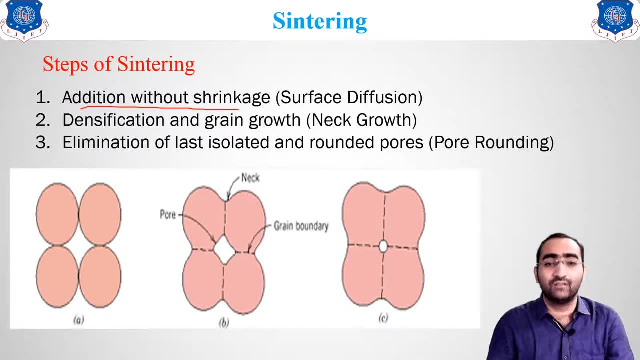 the thing. let us discuss it. the first one, that is addition without shrinkage. you can see, the particles will act individually: one, two, three, four, all the particles they are by the compression. they touch with each other. whenever the temperature increases, densification and grain growth take place, that means neck growth changes. so over here you can see there is a diffusion which is taking. 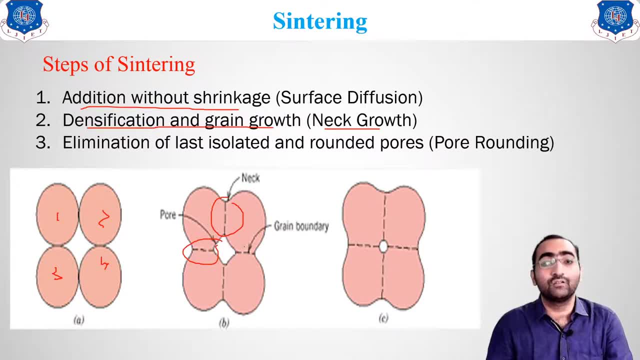 place. see the different layers, they are getting closer to each other. and contact surface- here there is. only this small amount of contact surface is there. here the contact surface has increased. and last one: elimination of the last isolated pores. that means pore rounding, means over here the gap, and now, as a result, slowly and steadily, the gap gets reduced, the void get reduced. so here, 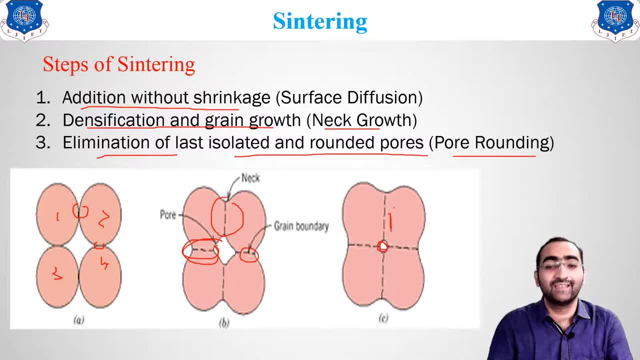 four particles will now behave as only single particle and, as i told you, after sintering the strength of the material is increased. why? because this four particle strength is less. if you apply load they will get disintegrated, but here it will not get disintegrated easily. large amount of 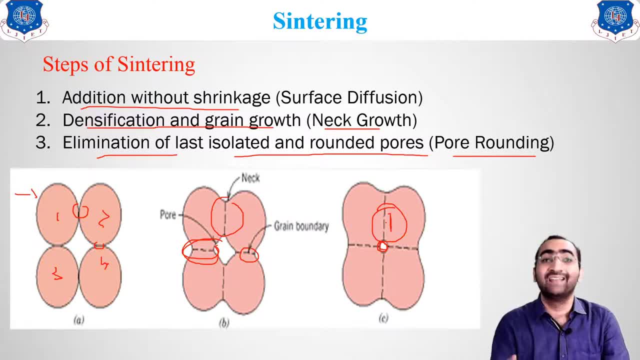 force is required for the breaking of this particle, and this is why sintering is very useful and as a result of which we are saying that powder metallurgy, they are having a high life and they are having a maximum strength, by which we are getting the maximum strength by this method. 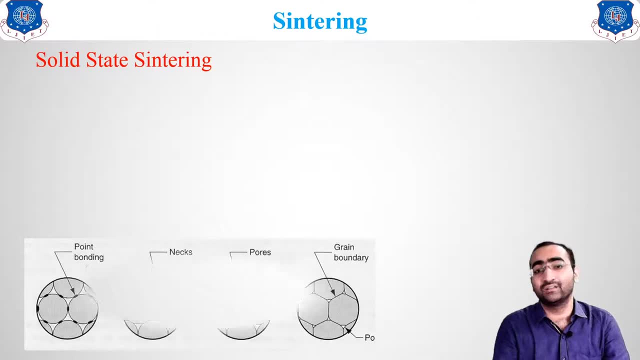 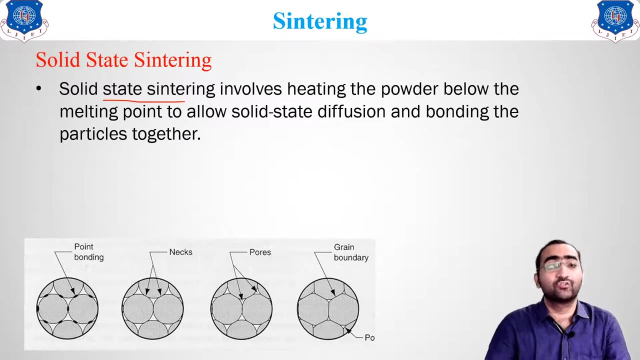 only let us discuss the two types of the sintering, that is, the solid state sintering. in that solid state sintering, what is happening for that sintering? you are saying that the solid state sintering involves heating of the powder below melting point to allow solid state diffusion. 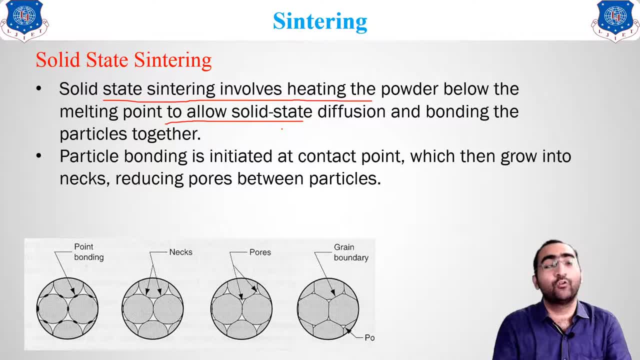 particles, bonding initiate at the contact surface and then the powder is released into the liquid point and they grow in the next and the particles will get around the boundaries. so here is the thing you can see: solid state sintering. whatever we discussed earlier in the steps, the same thing. 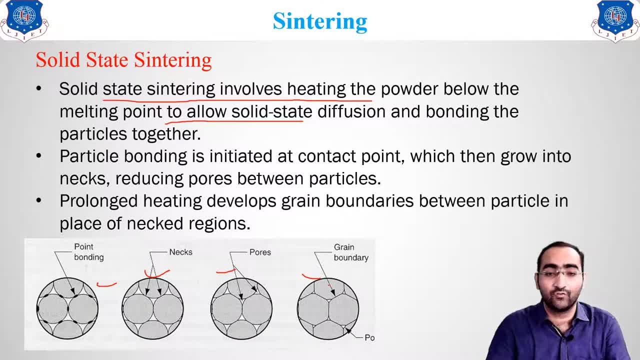 happens. over here you can see the different particles. and now you can see over here the different particles. that means your material in a solid state. if it is heated and if they are wetting close to each other due to that thing, what will happen? whatever the closeness is there in the solid, 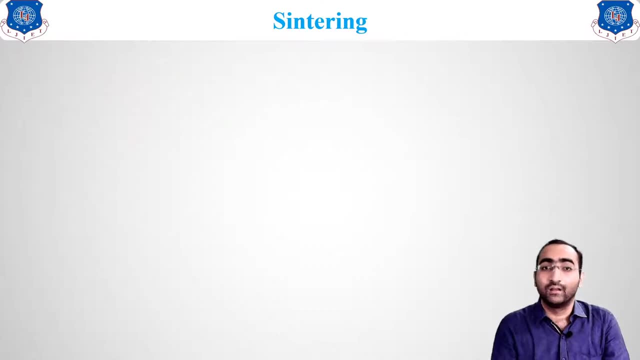 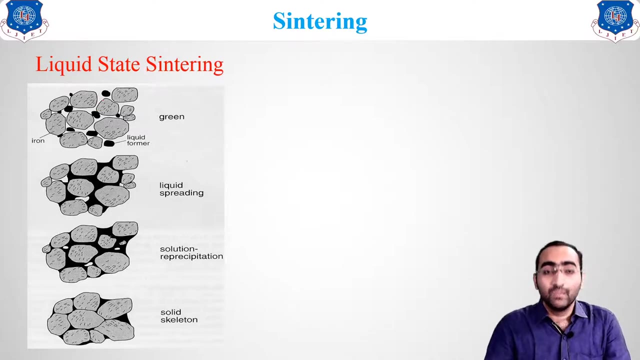 state. that is known as a solid state sintering. but there is a change in the liquid state sintering. what happens in the liquid state? we are taking the liquid material because in a solid state sometimes the voids which are there, they are remaining. 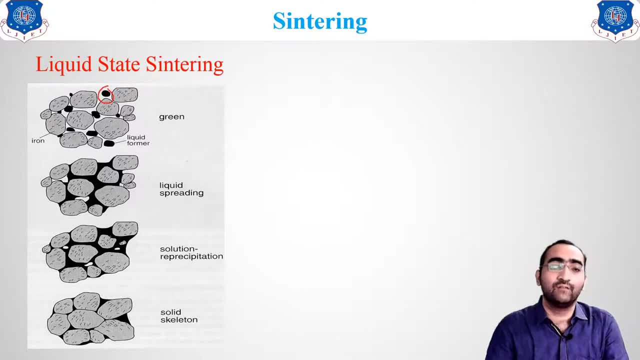 inside the material. so, for removing that thing, what we are taking, we are taking the liquid particles. when you will heat at that particular, this liquid- you can see over here- it will spread out in all the direction and, as a result of which, what we will get, the material will get. 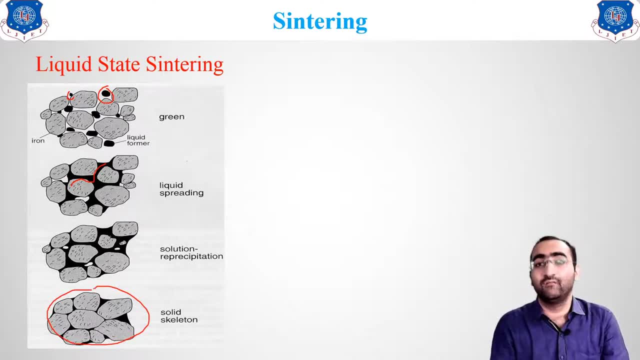 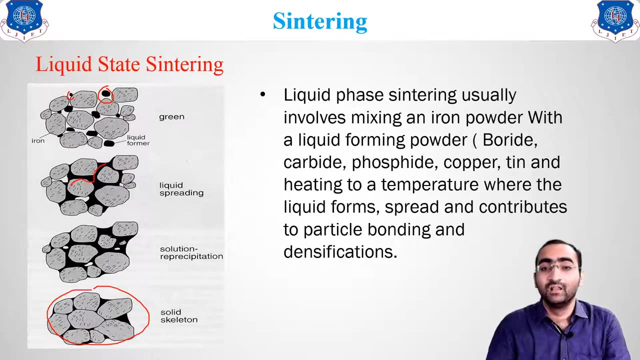 close to each other. so with the help of the liquid we are getting closer of the particles with the each other. so that is known as a liquid state sintering. liquid phase sintering usually involve mixing of iron powder with a liquid forming powder. liquid forming- they are the boride carbide firstly. 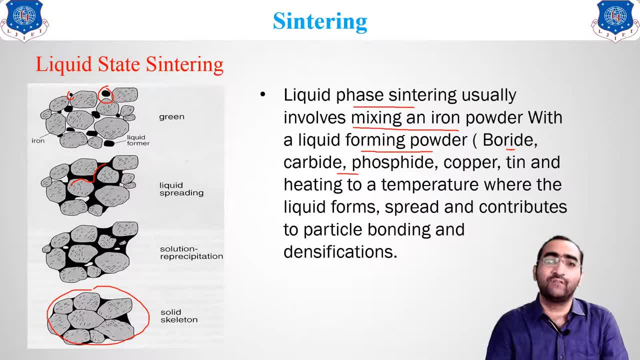 they are solid- here you can see. but as a small amount of heat is applied, they convert into liquid. so heating to a temperature where liquid forms sprayed and contributes to particle bonding and densification. so, as i told you, the liquid will get the particles closer to each other and they 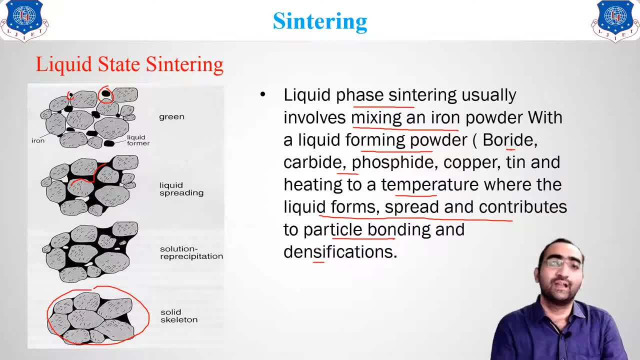 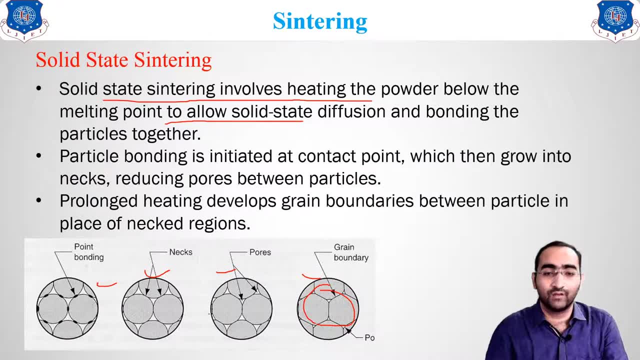 will bond with each other and, as a result, the material will get very close to each other. here, you can see, there is no thing which is left here. there is a thing which is left over. here, the small gaps are there small gaps, but in this thing you can see, there is no gap which is there. 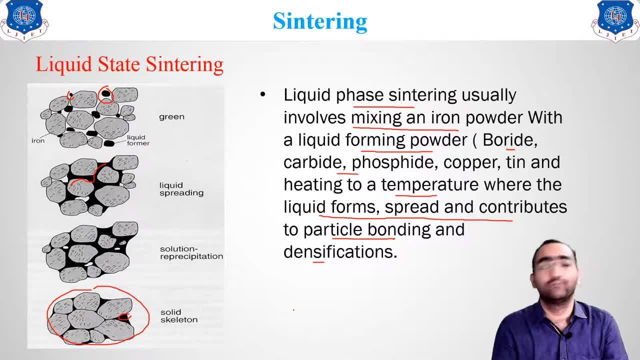 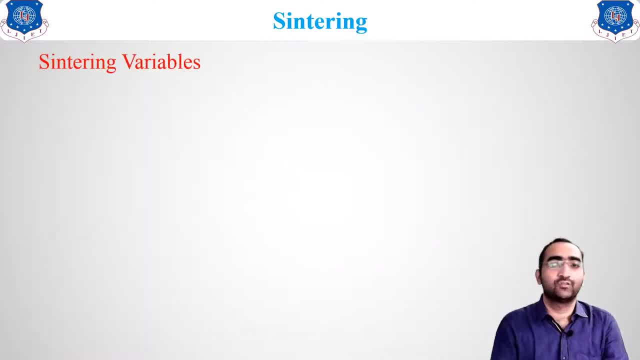 so strength of the material will be increased with the help of this sintering matter clear. so this was the solid state sintering and the liquid state sintering. so now let us go for the sintering variable on which the sintering depends. the very first one, temperature. as i told, 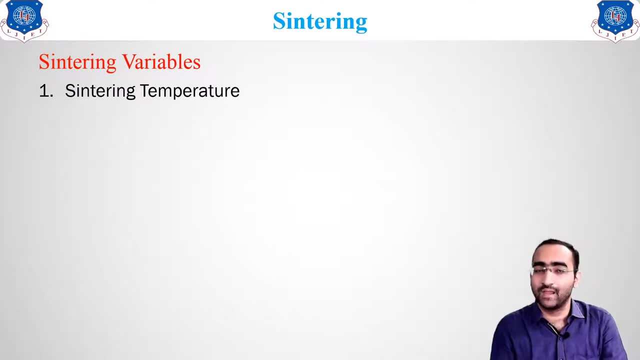 you. if the temperature is very much higher, liquid we will be getting, and that is of no use. if you are going for the low temperature- sintering, what will happen? due to the low temperature, proper bonding will not take place. so optimum temperature should be taken the same way time. if you go for 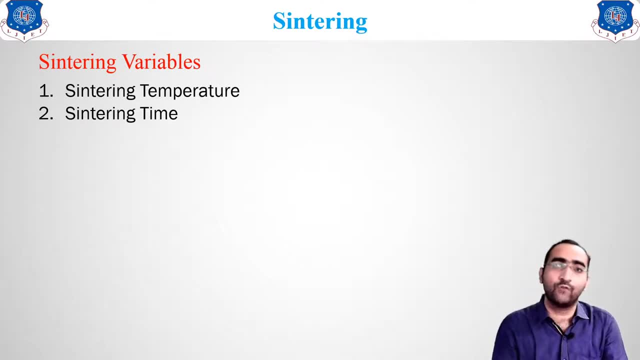 the more time burning sensation will there. if you go for the lesser time, proper bonding will not take place. so optimum sintering time is also used for the sintering process. and the third one, as i told you, the atmosphere, which atmosphere we are using the sintering depends on it. 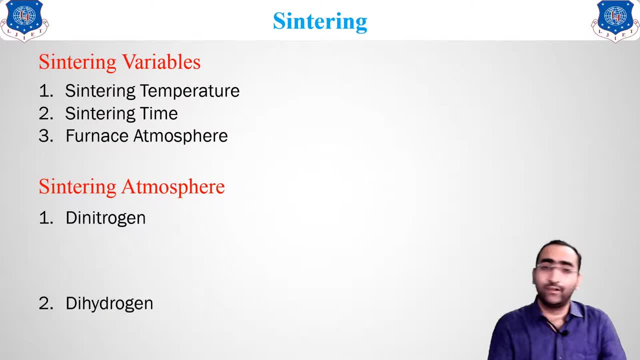 so which are the different atmosphere? we can use nitrogen. we can use hydrogen, ammonia, ammonia why? because hydrogen and nitrogen is only there in the ammonia vacuum. is there endothermic gases and exotherm? what are the endothermic gases? endothermic gases are the gases which 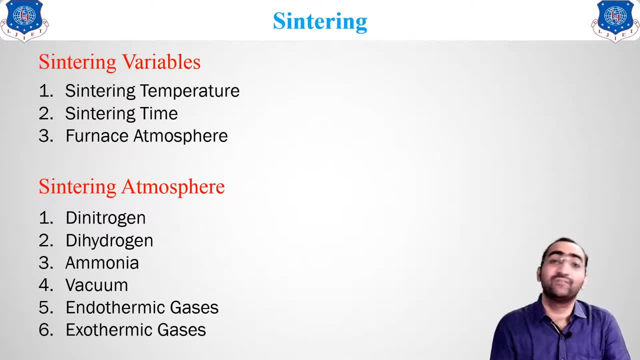 absorb the heat. exothermic gases are the gases which gives the heat. so these are the six of the different types of the atmosphere which we can take. we cannot do it in our normal atmosphere. clear, then, which are the zones of the sintering. there are three zones of the sintering. the first, 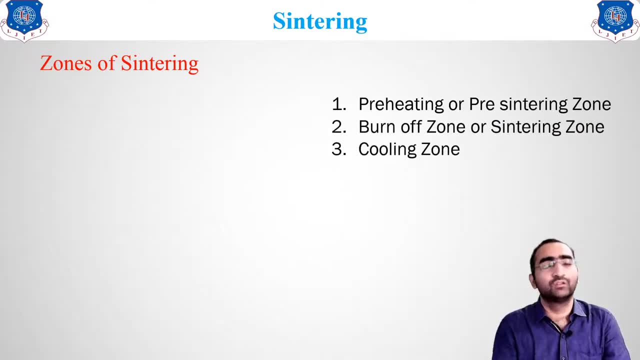 one preheating, second one burn off, third one cooling. what is this preheating zone? preheating zone is the zone in which only small amount of heat is applied so that the material gets acquainted with that thing. if suddenly a large amount of heat is provided, there are chances of cracks to followed. 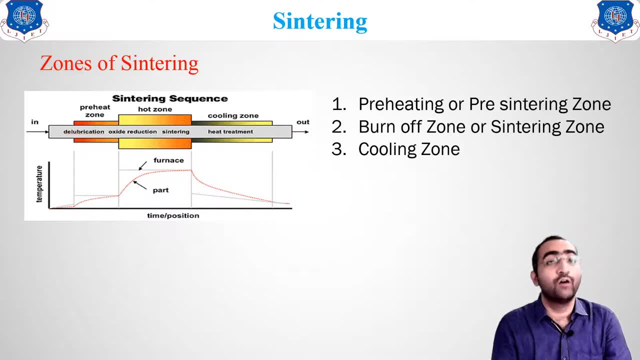 inside the material. so, for that thing, what will be happen? to avoid crack? what we are doing? we are going for the preheating. preheating or you can say pre-sintering, so that the material gets heat, they get familiar with the heat and there is no change in the property due to that thing after. 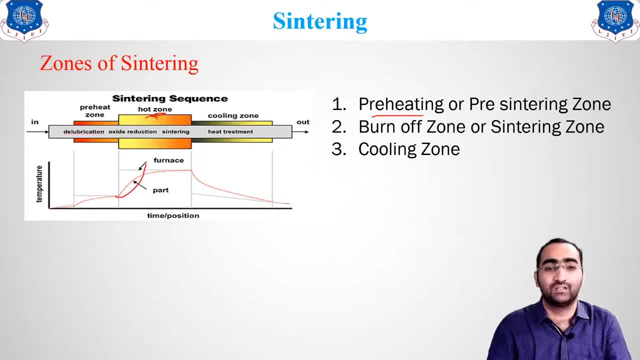 going for the hot zone. so you can see the temperature is increased and at last, in the furnace only it is allowed to cool to the room temperature. you can not go for the rapid cooling. why? because for the rapid cooling the material will be brittle, so inside the furnace only.